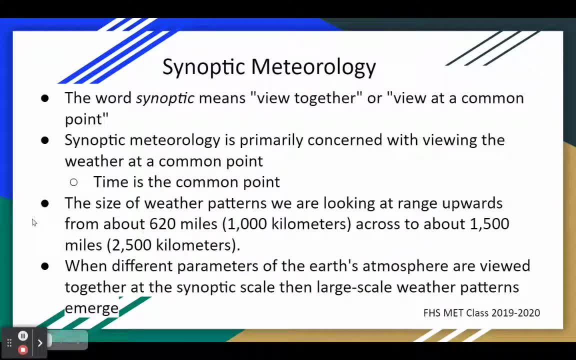 Okay. so when we talk about synaptic meteorology, the word synaptic means that we view it together or we view it at a common point. Time is the common point that we're looking at, And that's why we start this class this year with Zulu time, because Zulu time is the same time throughout the world. 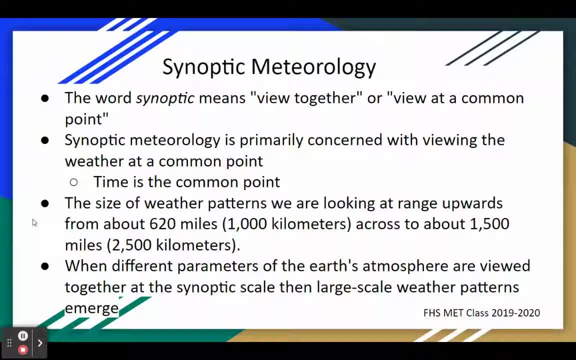 You still need to know which time zone you're in. For example, we're in the eastern time zone, So during eastern standard time we subtract four hours from the Zulu time, And in eastern daylight time we subtract five hours from the Zulu time. The size of the weather patterns we're looking at: they range upwards from about 620 miles to about 1500 miles, So we look at large weather patterns. 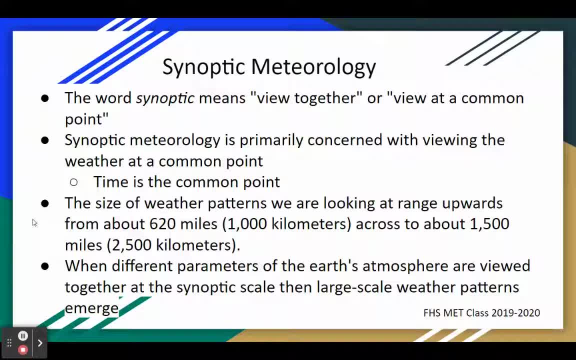 So we look at large weather patterns across the entire continental US, across the entire nation, And then, when different parameters of the air's atmosphere are viewed together, the synaptic scale then creates these large scale weather patterns which help us with the predictions that we make. 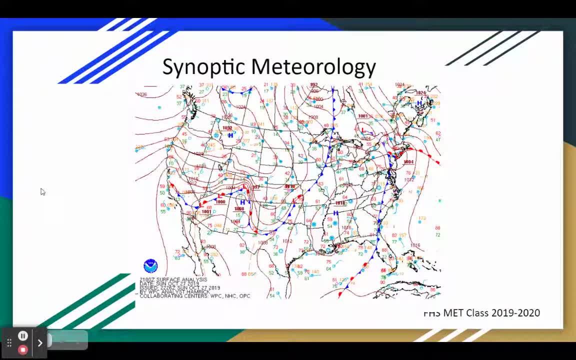 Okay, so here's a US, continental US weather map And you can see there's different symbols on these weather maps. So just to look at a few of them, We have low pressure, We have high pressure, We have numbers next to these pressure systems: 1032, 1001.. So the pressure in millibars. We also have different fronts that we'll get into and talk about Cold fronts here, warm fronts over here. So those fronts help determine our weather also. Now think back to the last unit that we talked about also when we talked about the westerlies or the winds that blow in the US. 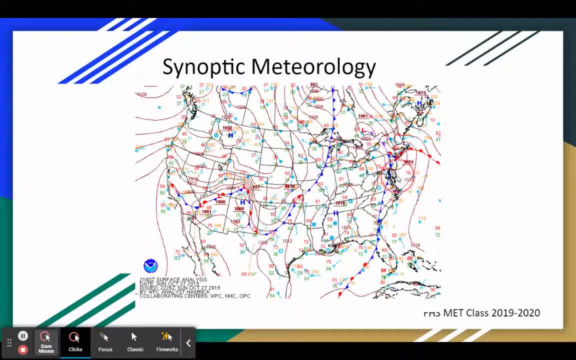 These weather patterns tend to move from one direction to the other. So we look at a few of these weather patterns across the entire continental US. So we look at a few of these weather patterns across the entire continental US. So if we have low pressure just focusing on Michigan, if we have low pressure near us now, this low pressure system is going to move to the east and will eventually be replaced by this high pressure. 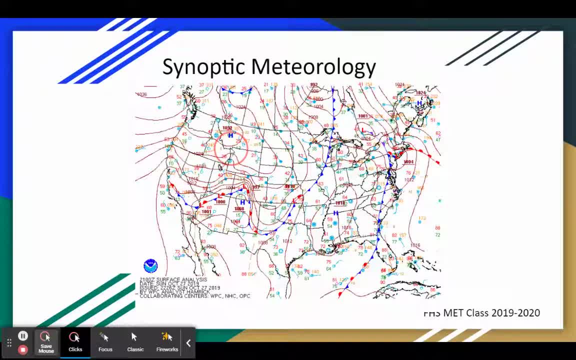 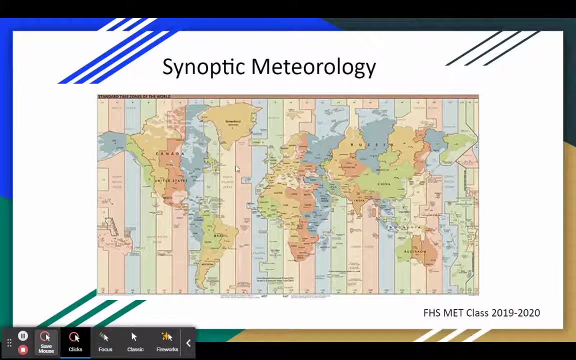 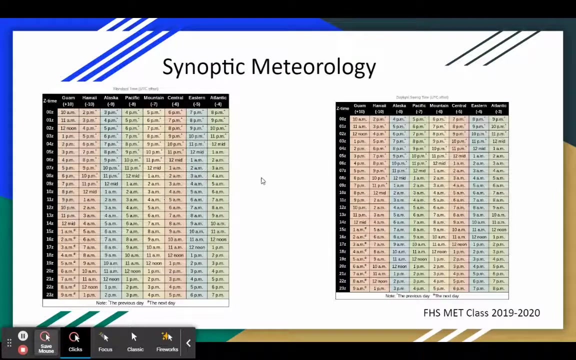 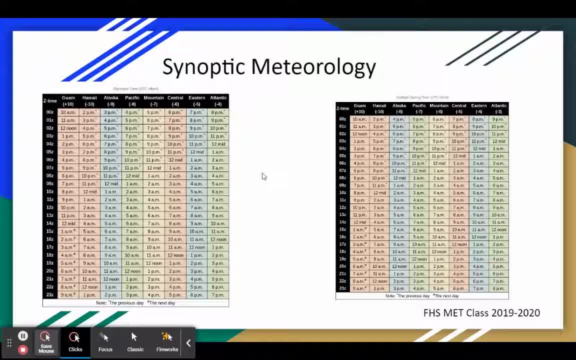 by daylight savings and by standard time. So right now we're in daylight saving time mode. After the beginning of March we switched to daylight saving time And in the eastern time zone again we subtract four hours during daylight saving time. In the fall when we go back to standard time or EST eastern standard time, we then subtract five hours to determine the zoom time. 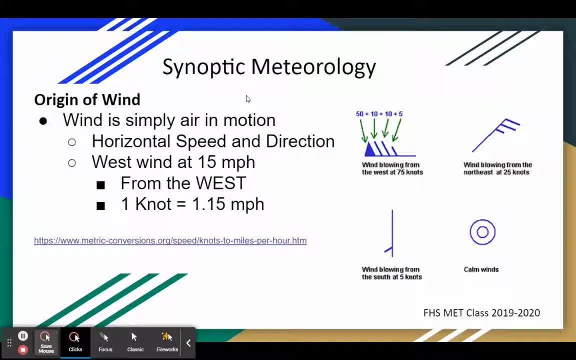 okay, so here's a little um bit of review, but also maybe a little bit of new stuff. we looked at a little bit of high and low pressure and how that determines our wind and wind direction to wind speed. but the origin of wind is that wind is simply air in motion. we can measure the horizontal 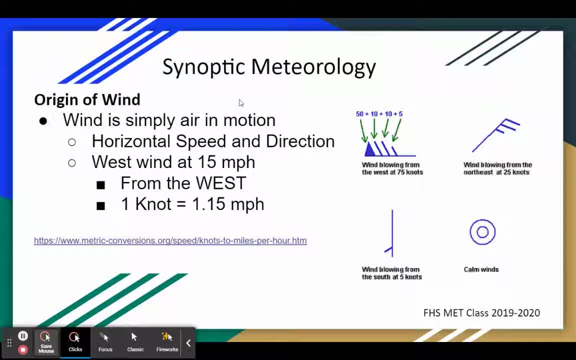 speed and direction of the wind, and remember that we always give the wind direction from where it's coming from. and then just a conversion here, because we're more used to miles per hour with driving and anything else we do. um, they, they give the the speed of wind in knots on weather maps. 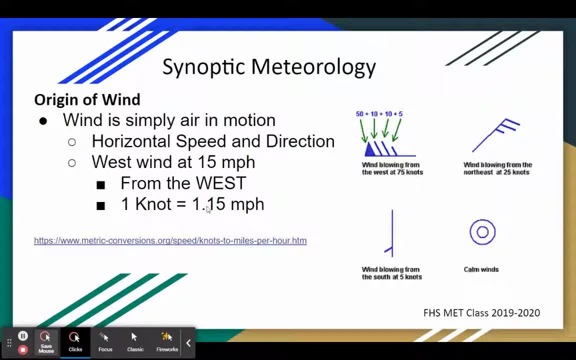 so to convert from knots to miles per hour, they're they're pretty close, but one knot. you would multiply that by 1.15 to determine miles per hour, or one knot equals 1.15 miles per hour. okay, so if we look at this, because you'll, you'll view these on weather maps also- this right here again. 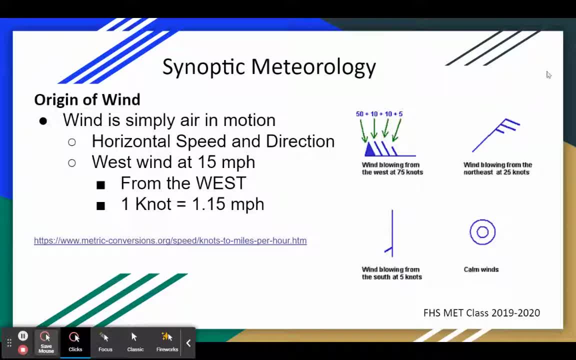 we. we determine wind by where it's coming from and we go through the feathers into the circle or into the station model. so these winds right here are coming from the northeast. if we look at a northeast- southwest compass, so they're coming from the northeast. and then to determine the 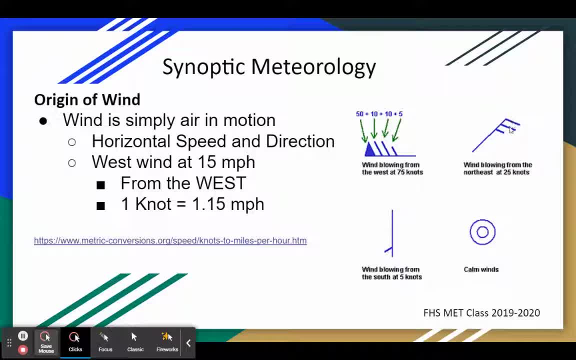 number of knots. we're going to go through the feathers and then we're going to go through the Zeus breath area and then we're going to add up these flags here- 10, 20, 25- and then here's a description of what all these flags mean again. so if we look at this weather Station model, right, 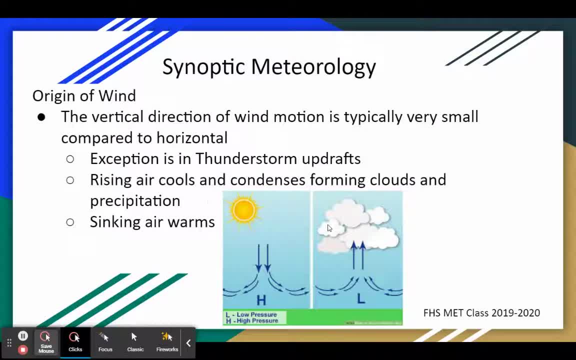 here the winds are coming from the south at five knots. the vertical direction of wind is small compared to the horizontal and where low and high pressure coming to play. okay, the exception to this is that sometimes thunderstorms will have very strong up up drops with which the wind is raised否. have very strong up drops with which the wind is raised. all you're going to run in this direction is very strong up to. you're going to learn first. one is: not only is the spokesman told you about, you're noting all your Hazard states makes you. however large are airilanche flat, you have 3,000 dollars, a Messi or two large. 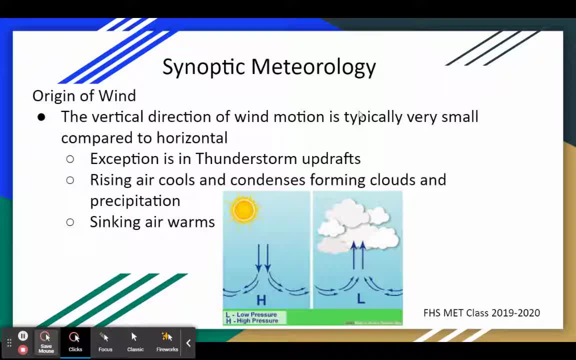 asted. you know some number and the data set you want to use. the провод is well understood. okay, you can catching up it. I need a updrafts or downdrafts. Rising air cools and condenses. That's how clouds and precipitation 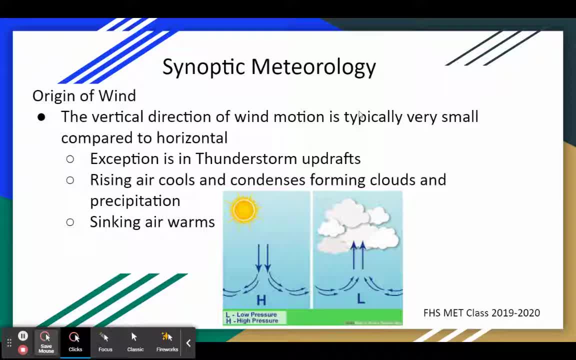 form and sinking air warms. So we can compare it to this weekend. this weekend, especially yesterday, very cloudy, rainy, some snowflakes mixing in, and also very windy. That was low pressure over us. Low pressure is air rising and being replaced by or actually flowing. 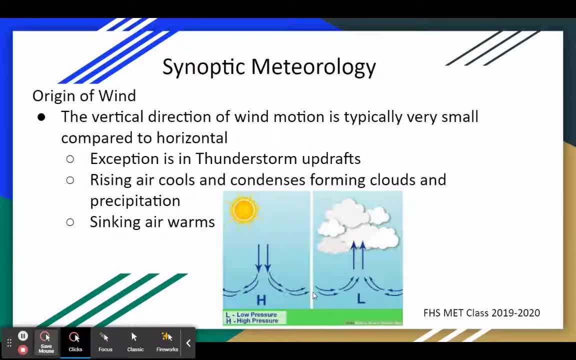 this rising air is replaced by high pressure, most likely to our west, flowing in very quickly. That air rises and forms clouds to form or causes clouds to form. During high pressure, the air sinks and because it sinks it's being pressed towards the ground. that most likely. 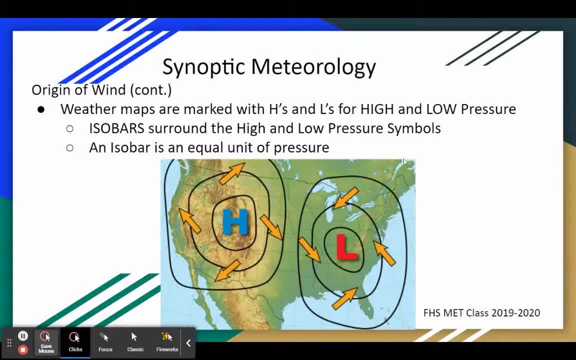 like today, causes sunny skies. Okay, so here's a weather map with both high and low pressure on it. Remember what we talked about with the Coriolis effect and why things spin the way they do in the northern hemisphere, But on this weather, 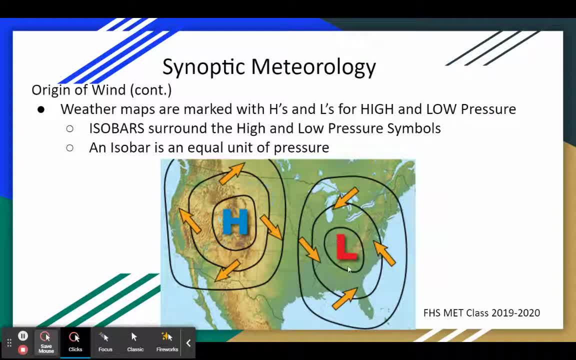 map. we have low pressure and high pressure. These lines around the pressure systems are called isobars. These isobars surround high and low pressure, and an isobar is an equal unit of pressure. So, along this line, right here, along this line, right here, all of this along this line. 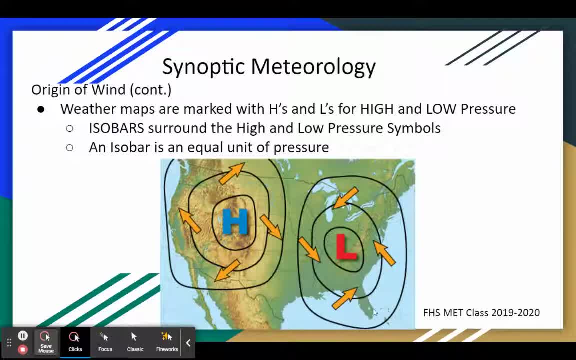 is the same pressure, And this would be lower pressure because we're approaching the low pressure. but all of this along this line is the same pressure, It's just lower than this. All of this along this isobar is the same pressure, but it's lower than these other two. And then, with these lines, again same thing. 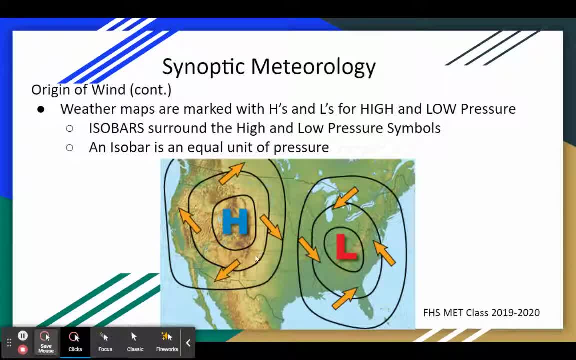 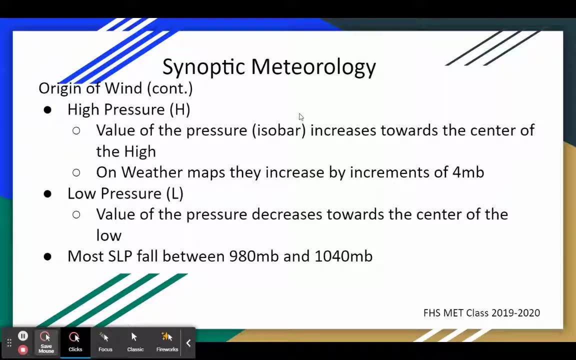 an isobar connects areas of equal pressure. As you go into the high pressure or get closer to the high pressure, the pressure along these isobars rises. Okay, so high pressure pressure: the value of the pressure increases towards the high On weather maps they increase. 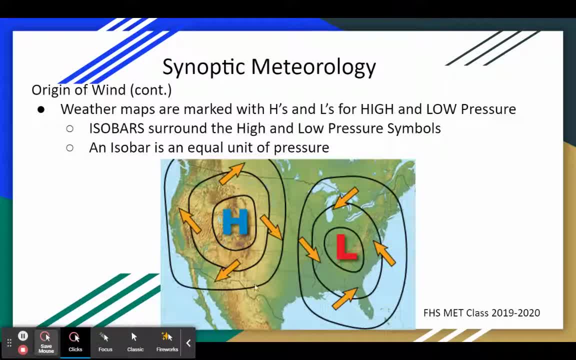 by increments of four. So if we go back to this right here, if this is 1,000 millibars, this one would be 1,004.. This one would be 1,008 millibars, increasing as you go into the high If we decrease. 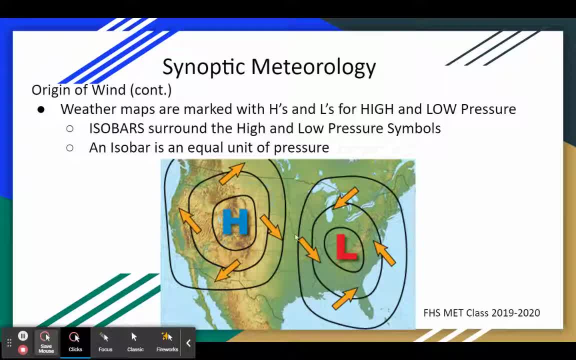 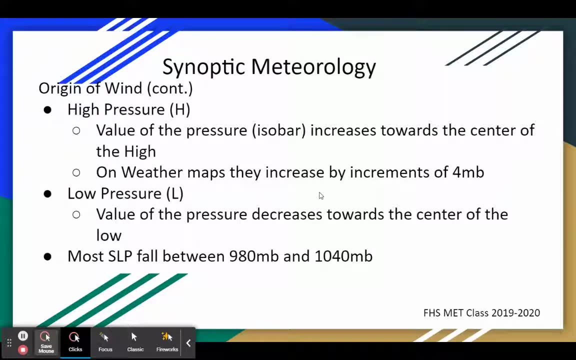 as we go into the low. if this is 1,000 millibars, this would be 996 and 992.. So decreasing as we go towards the low Most sea level pressure that we look at, and we talked about this when we 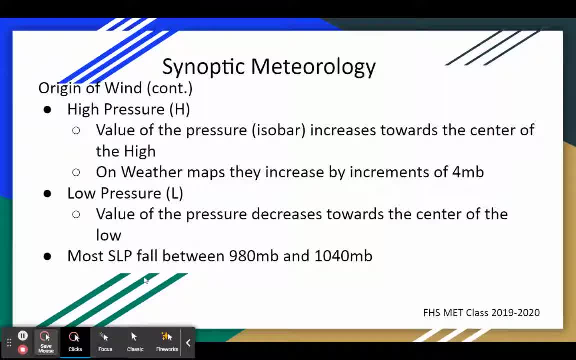 converted station model pressure, but most of the sea level pressure falls between 980 and 1040 millibars. Anything below 980 is a very low, low pressure system And anything above 1040 is a very high, high pressure system. 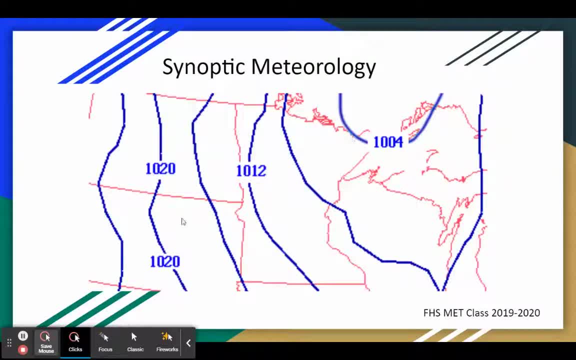 Okay, so here's those isobars again and the increase by increments of four. If this is 1,004,. if this isobar is 1,004 millibars, this one would be 1,008,, 1,012,, 1,016,, 1,020, and 1,024.. 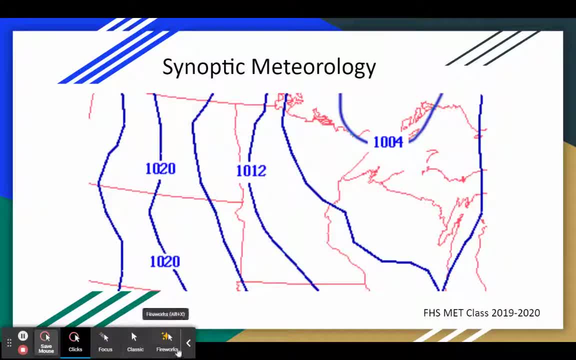 You may need to highlight these. You may need to highlight these on a map- And I'm actually trying to pull up there it is- So you may need to not highlight, but you may need to label these on a map And if you had to again, they just increase by increments of four. So either approaching 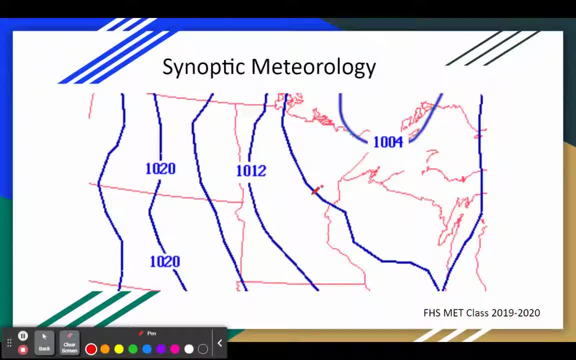 the high pressure or approaching the low. So here's 1,004,, 1,008,, 1,012,. this one would be 1,016,, 1,020, and 1,024.. Now, also, if they ask you to label where the low 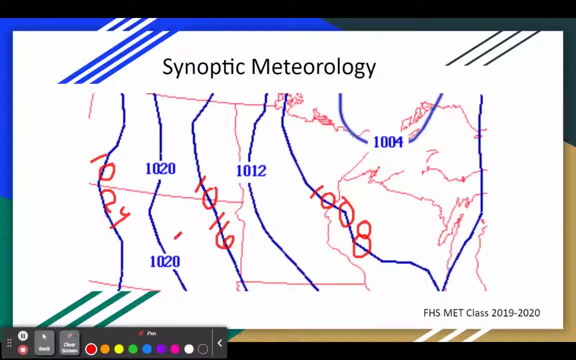 pressure system is. remember that the pressure drops going into the low. So just look at this map right here. You should be able to label where the low pressure is on this map And it would be right up here. Okay, And if we were to label this isobar, this would be 1,000 millibars. 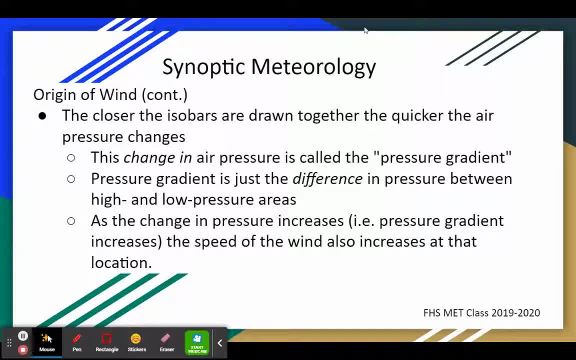 The closer the isobars are drawn together, the quicker the air pressure changes. Or to put that simply: the closer the isobars are together on a map, the windier it is in that area. Okay, The change in pressure is called the pressure of the air pressure. So if we were to label this, 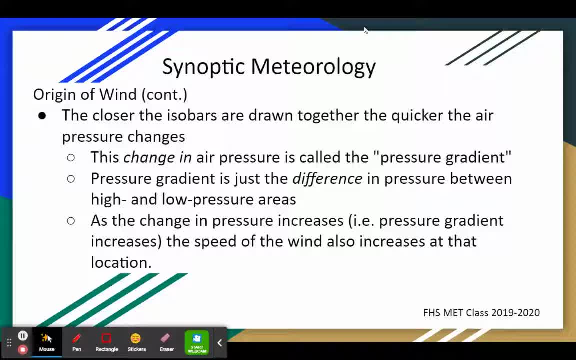 as a pressure gradient. if the pressure gradient is changing very quickly in a smaller amount of time or a smaller space, that creates a pressure flow or more wind. Pressure gradients just the difference in pressure between high and low pressure And as the change in pressure increases. 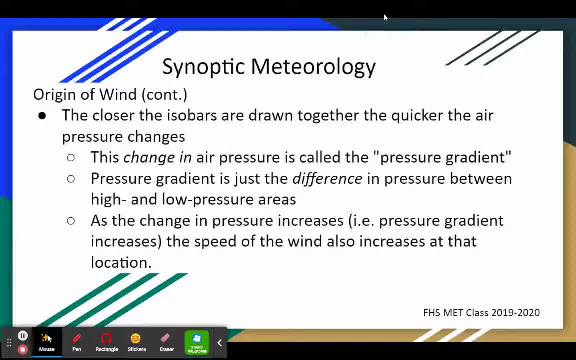 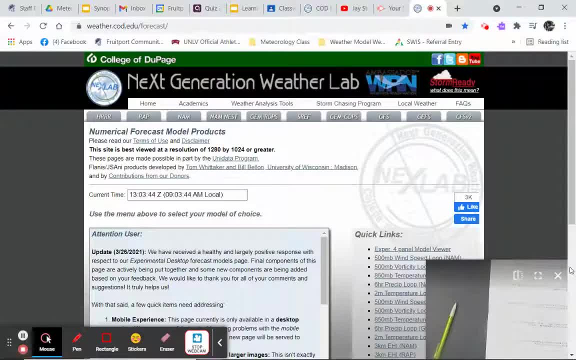 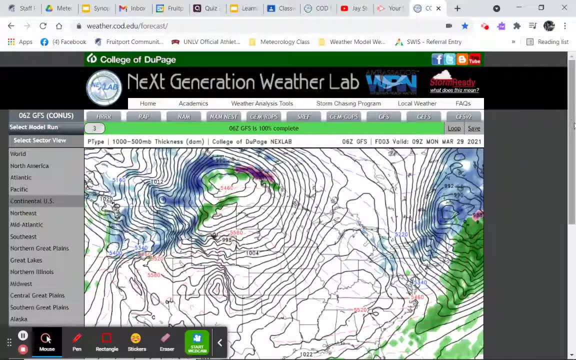 the speed of the wind also increases at that location. So let me show you that in real time. right now We go to this College of DuPage site And we'll just go GFS and the Continental US And you can see here, if you're looking at this map, 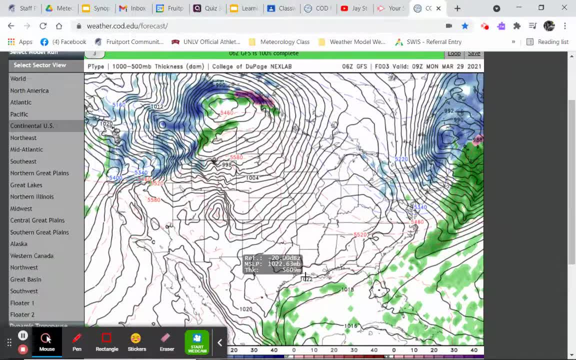 right here, where the windiest part of the map is. Okay, Remember these isobars. right here, where they're closer together, is where the windier part is. So they're closer together right here. It's windiest right here And it's windiest out here, where they're close together. 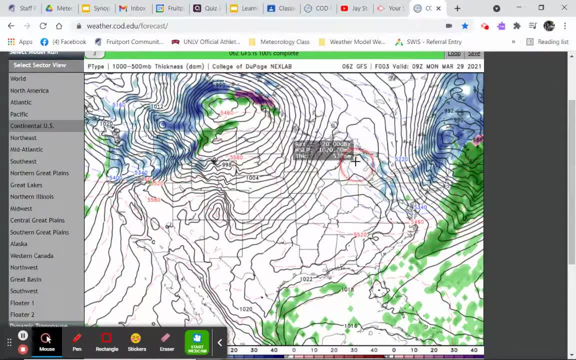 Where we are in Michigan today we have a little bit of a break from the winds from yesterday. Okay, Here's that low pressure from yesterday moved out. Here is- let's see another low pressure system out here, And this is high right here And you can actually look at this. Let me. 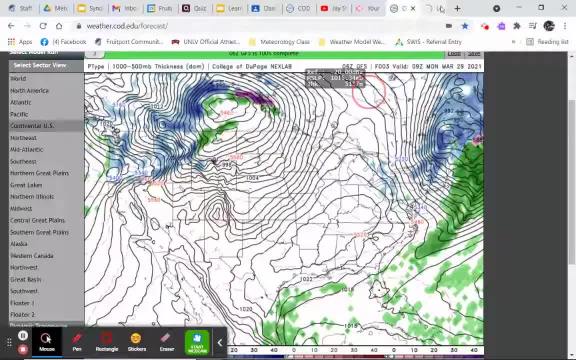 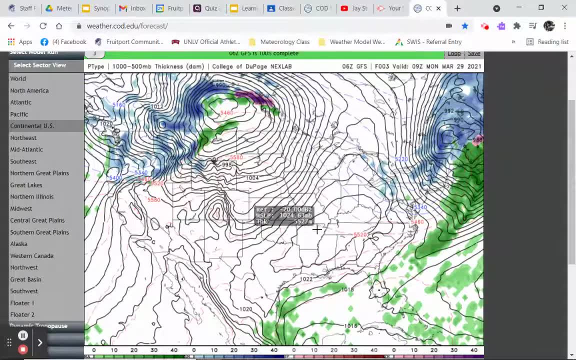 get rid of this little mouse right here. What the let me get rid of this little mouse right here, Okay? And then, if we place our our cursor over this map right here, this is 1025 millibars. Watch as I move away from it. 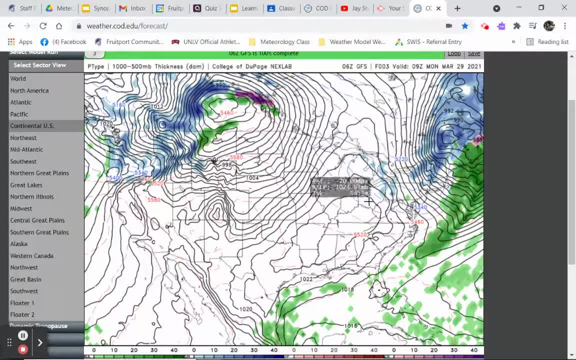 it drops all the way up to 985.. And then again 1025,. as we move away from it, it drops to 982.. So we're actually in the middle of two very low pressure systems And we have high pressure overhead or close to us, where we are right now, And that's bringing the sunny weather that we have. 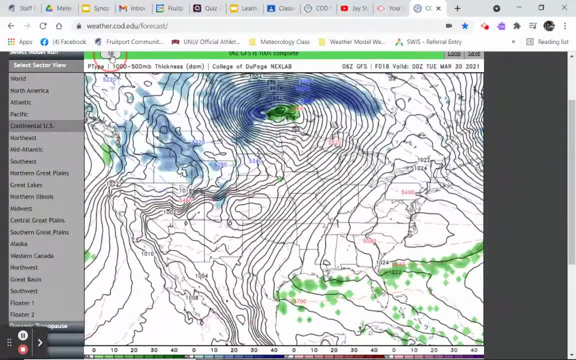 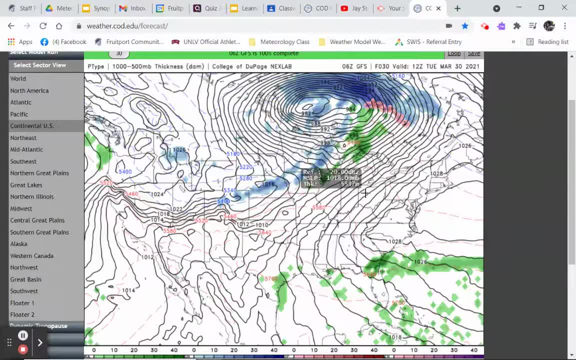 It's occurring today. So watch as we move forward here And then as you look at going through tonight into tomorrow, what would you expect the winds to do? And if you said, increase, that is correct. Here's the low pressure. This is a low pressure system. Look, it's 979.. So that's a very 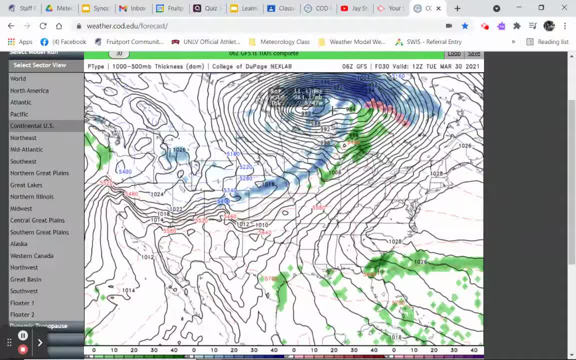 low pressure system. You can see the very strong winds up here and actually all around this low pressure. Here's high pressure in between the two pressures And then you can see the winds up here And then you can see the high pressure systems is where we're getting the wind. So low pressure. 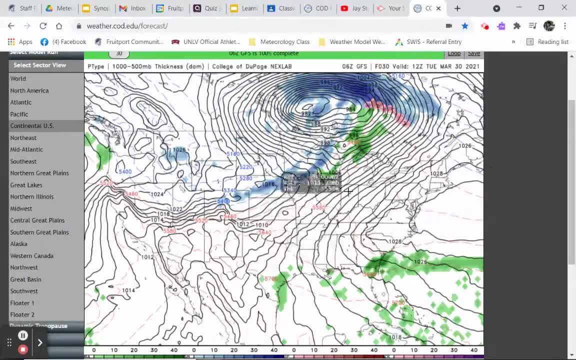 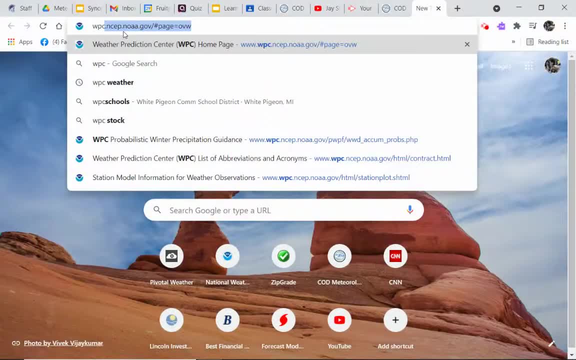 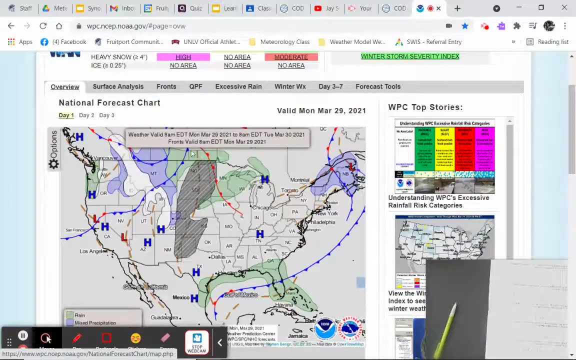 spinning counterclockwise, high pressure, spinning clockwise, and here's the winds in between. So this is tomorrow morning, Tuesday morning, And if we actually look at a map right here, you can see low pressure, high pressure and then that low pressure. 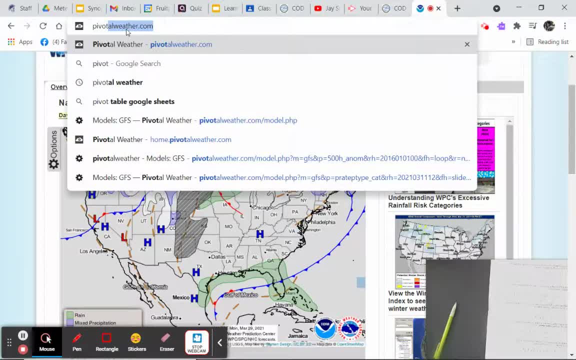 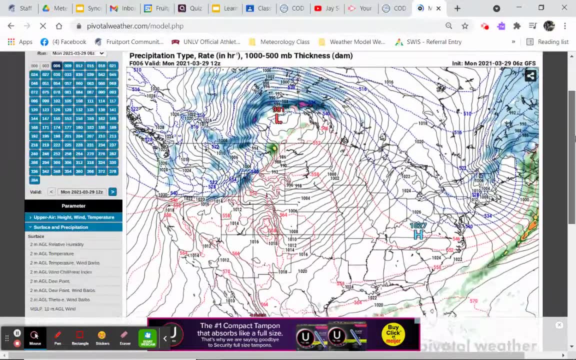 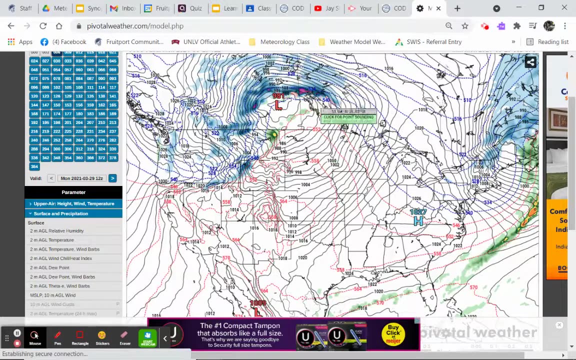 So these have those labeled on them. Another good one is the pivotal weather one. And going to the models GFS, and here they are, right here, The high pressure over us today, low pressure that was over us yesterday and then the low pressure up here. So this, actually, 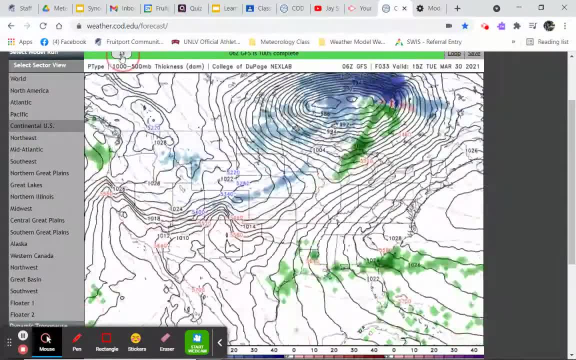 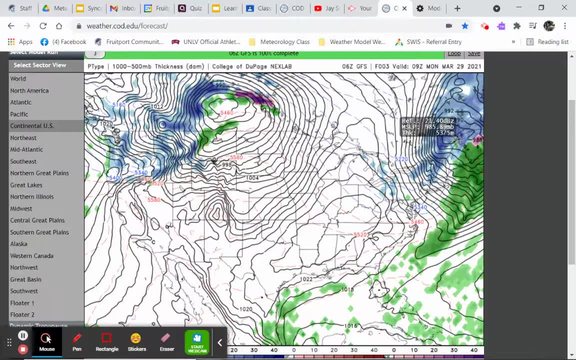 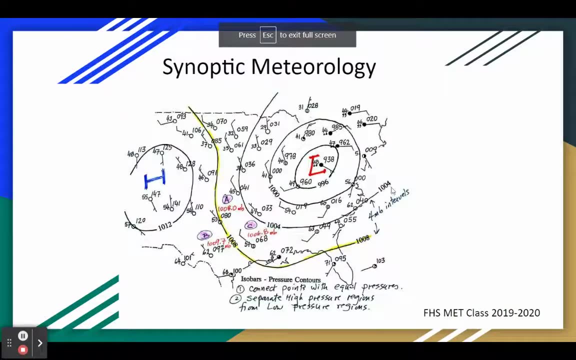 labels the pressures for you, The COD, the College of DuPage site. you just have to put your cursor over it and it will tell you the pressure systems. Okay, Here's another map with low and high pressure labeled. Remember, low pressure spins. 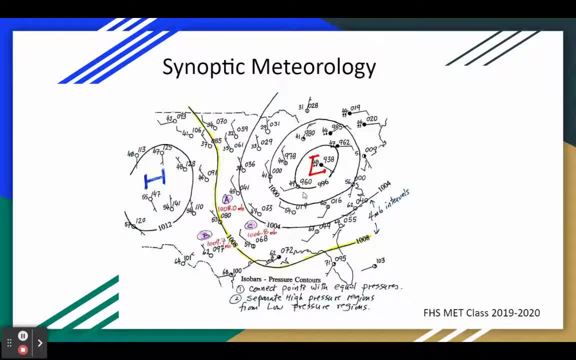 counterclockwise. And here's another thing to look at. here You can actually see the wind directions change around the low pressure. Okay, Because the low is spinning counterclockwise. winds from the northwest over here, winds from the southwest over here, winds from the southeast. 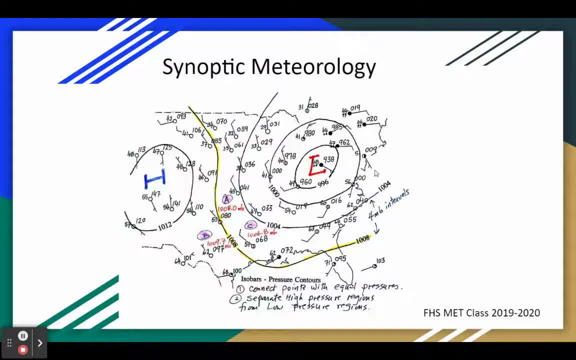 and north, northeast and north. So the winds also change around that low pressure system, Around that low pressure, And then you can actually see the wind directions change around the low pressure high pressure system. it spins clockwise and you can see the winds changing around the high pressure. 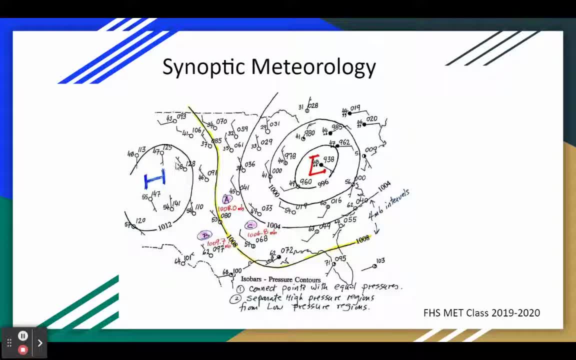 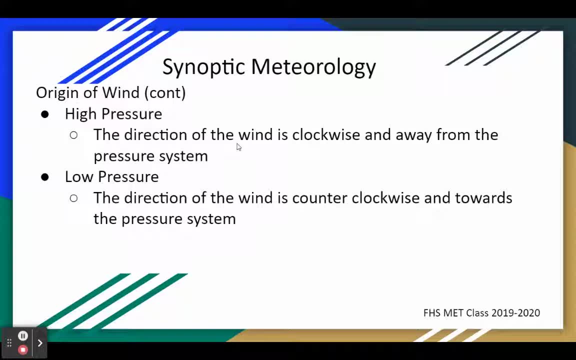 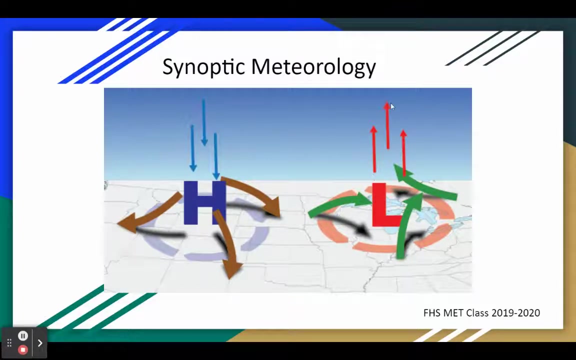 system clockwise. okay, high pressure- here's what we just talked about. we kind of been focusing on this. high pressure: the direction of the wind is clockwise and away from the pressure system. low pressure: the direction is counterclockwise and towards the pressure system. and then here's another model showing the surface: low pressure, spinning counterclockwise and rising. 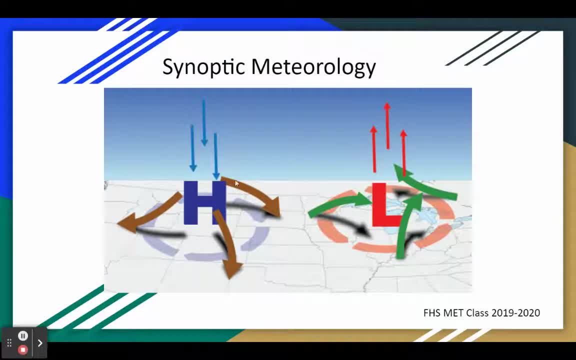 high pressure being pushed away, clockwise forced down and being pushed out. so, as this air is rising, the low pressure this air being forced down flows into it and it creates a convection current rising, sinking flowing. remember even when we talked about seeing land breezes: the air flows from high to low. 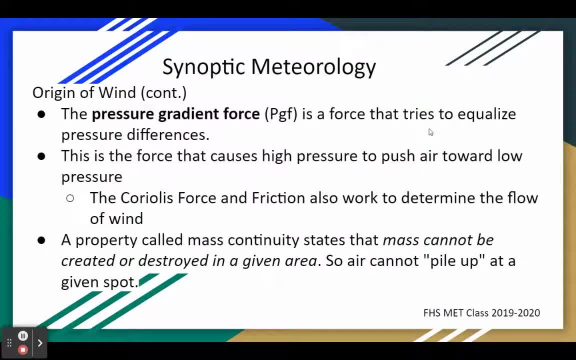 pressure. okay, a couple other things to end. with the pgf, the pressure gradient force, is that force that tries to equalize pressure differences and that's why, as it's flowing from high to low, we get those strong winds. this force causes high pressure to push towards the low. 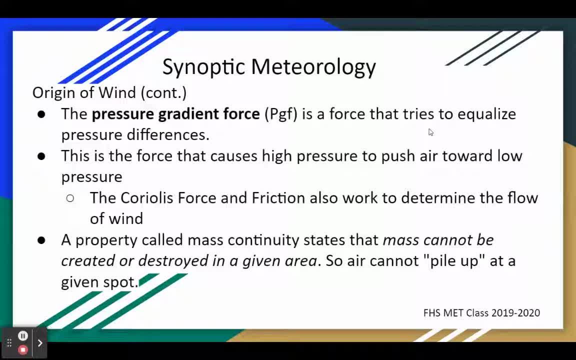 the coriolis of four, the coriolis effect, the coriolis force and friction determine the flow of the wind. and then that property of mass continuities just states that mass cannot be created or destroyed, and that's what we're talking about here. so that's what we're talking about here.